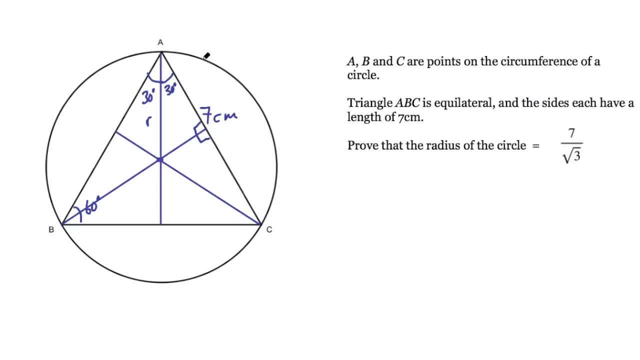 So, using this setup, that's going to help me solve this problem. Something else I can state is: because this is a 30 degree angle and this is a 90 degree angle, this angle in here must be a 60 degree angle. So what I have here is a right angle triangle with an angle of 30 degrees. 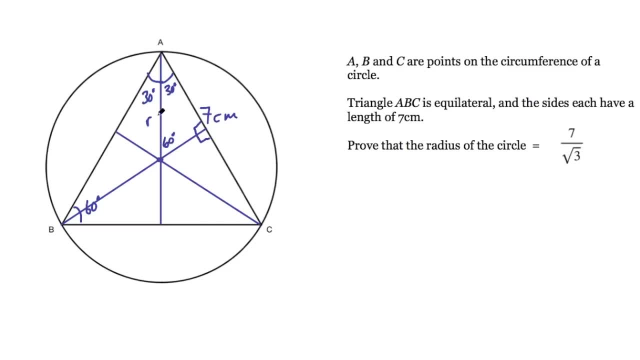 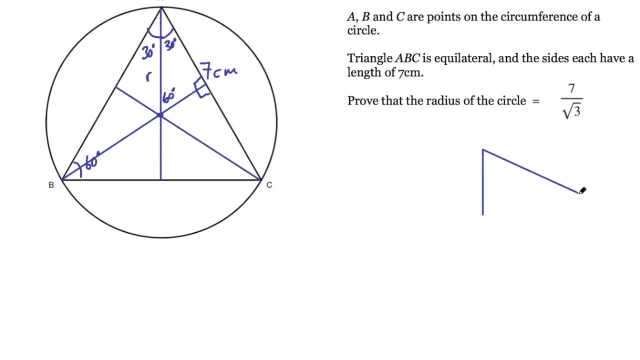 and an angle of 60 degrees, And I actually know something about the ratio of the sides of a right angle triangle like this. So if I draw a quick right angle triangle down here and the angles are 30 and 60, the ratio of the sides of this triangle 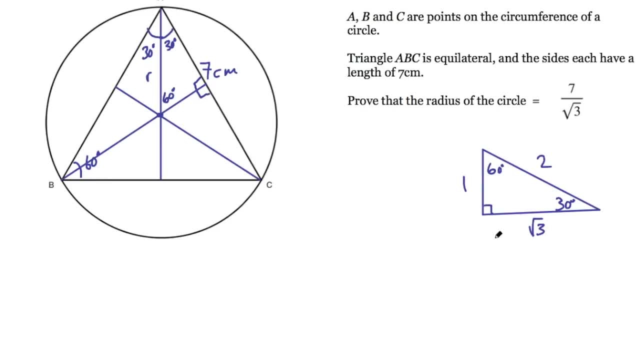 are 2 to root 3.. This is commonly used in trigonometry when talking about the sine and the cosine of angles, So this can often be used in problems like this, and this will allow me to find the radius. The other thing I can say is: 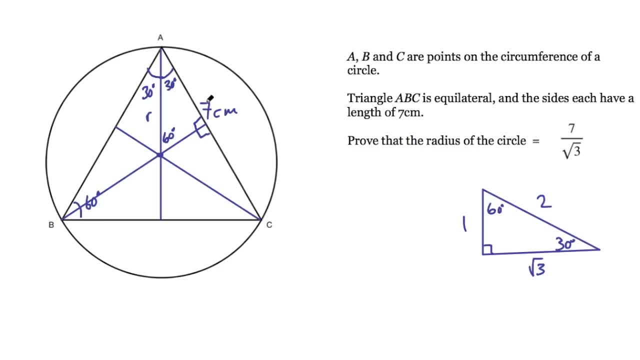 because this, this line, is cutting this angle in half. it's also cutting the length of the triangle in half. So this line, from point A to the center of this line, let's call it D, this line, AD will be 7 centimeters. 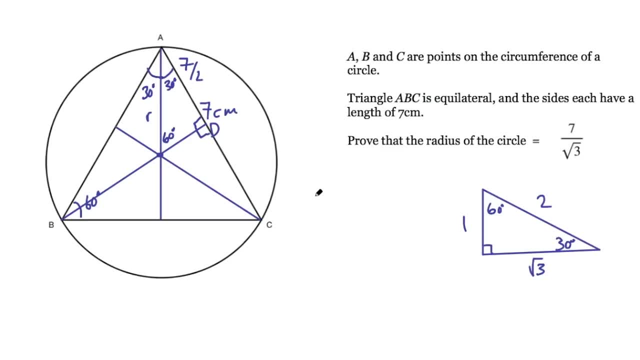 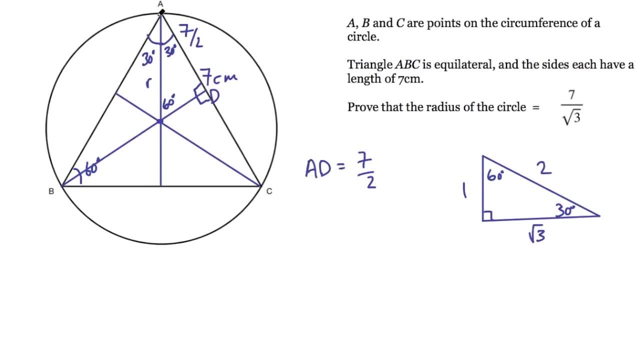 divided by 2.. So I'll write that as seven on 2.. So I know that AD equals 7 on 2.. And I know the ratio of the radius of the hypotenuse of this right angle triangle to this leg, AD is. 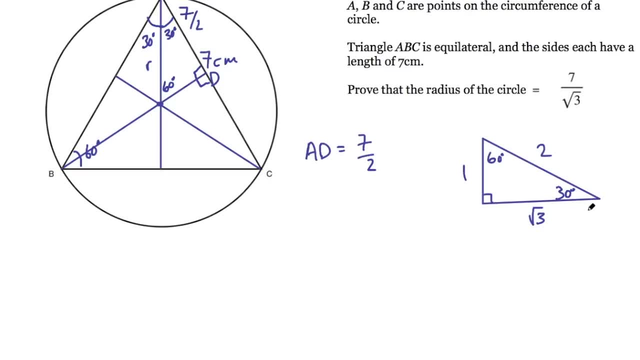 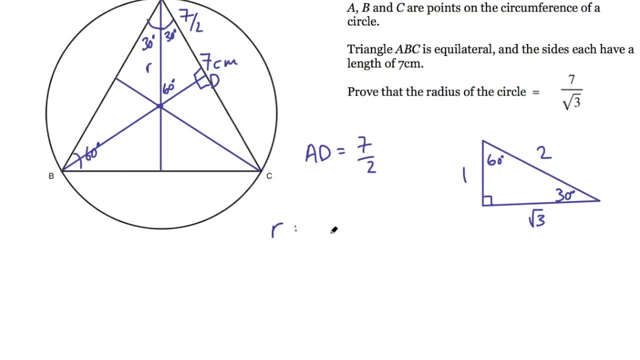 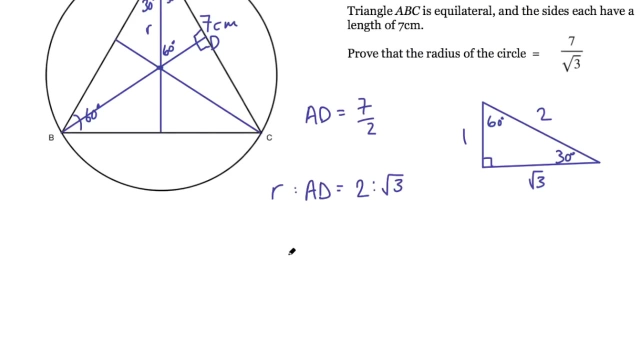 2 to root 3.. So in this diagram the bottom edge is root 3 and the hypotenuse is 2, so I can say the ratio of the radius to this edge, AD, equals 2 to root 3.. Now I know what AD is, so I can say the ratio of the radius to AD is R to 7. on 2. 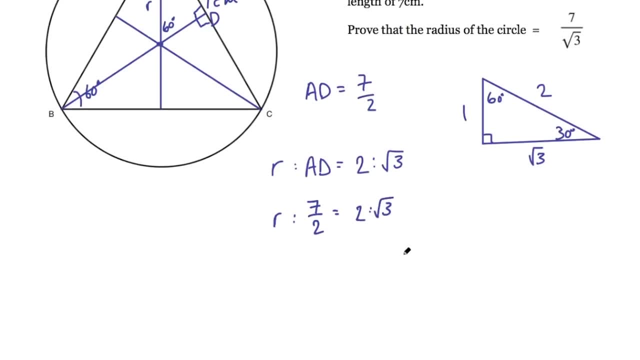 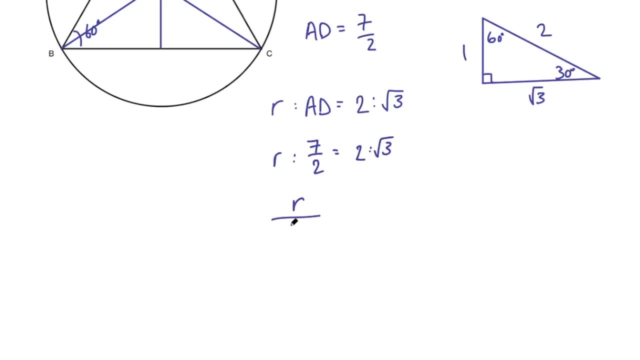 equals 2 to root 3.. And now, if I rewrite these as fractions- remember, you can always write ratios as fractions- I can say that R divided by 7 on 2 equals 2 on root 3.. So to get R by itself, I need: 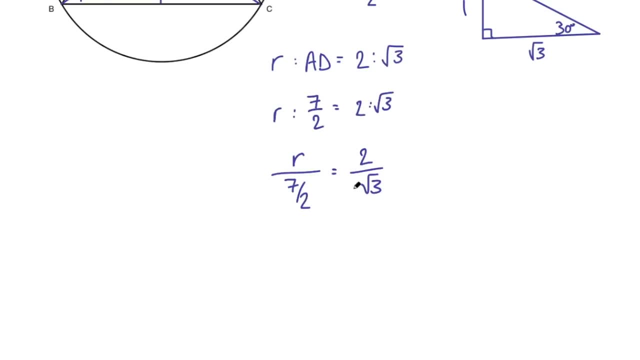 to multiply this side by the denominator. so I need to multiply the right hand side by 7 on 2.. So R is going to equal 2 on root, 3 multiplied by 7 on 2. And here I'm multiplying fractions, so I